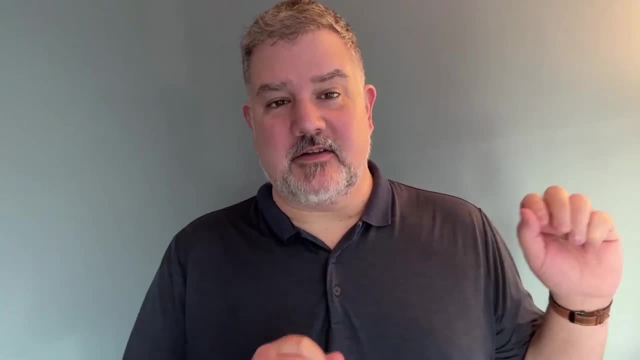 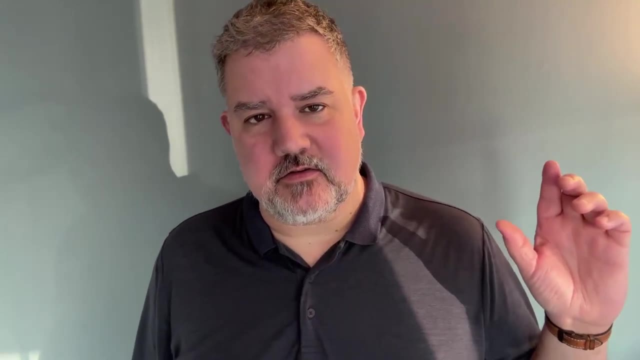 that they're using the spreadsheet in, or whatever into their database, and today that's what we're going to take a look at Now. if you're on my Patreon, make sure to check out my latest video, where I talk about why data normalization is so important. Let's get to it. 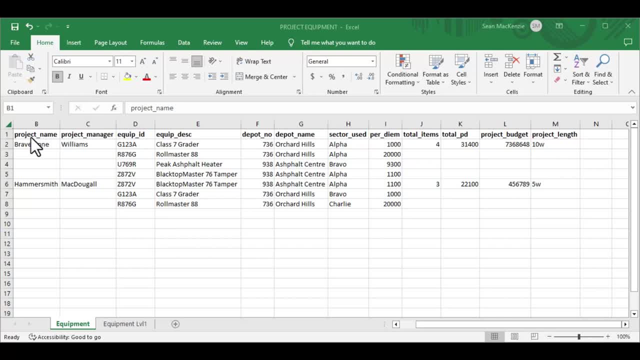 Okay, so most examples that I have seen start with a spreadsheet, and usually it is some data that has been collected manually and people are managing some process in a spreadsheet and eventually it gets too big for the spreadsheet and they go. well, hey, can we create a database and 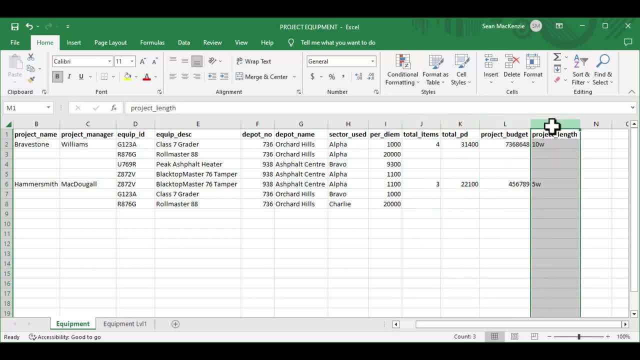 then an application that will handle this, and so, as you can see in this spreadsheet, I have a project with a whole bunch of equipment that's being used on a particular project, and you can see there's two projects: there's a bravestone project and a hammersmith project. 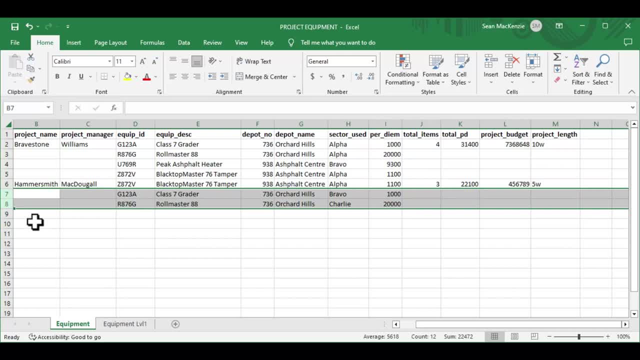 and it looks like there are some empty rows here, and so you get a sense that we need to figure out what this data means. and, upon closer inspection, we can see that there is a project group and you can see in the project group- there, you know, there's a name, there's a. 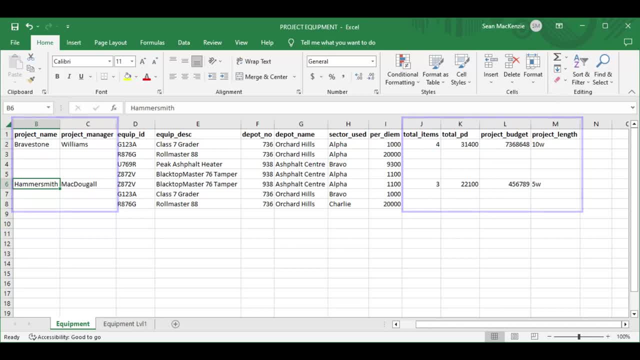 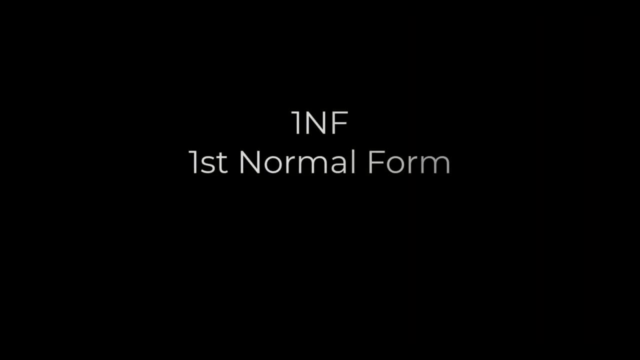 manager and you know project length and things, and then there's also almost like an equipment list for each of those projects, and you know, this looks like it's a sample from a much bigger spreadsheet that has way more entries on it, and so that takes us to our first task, which 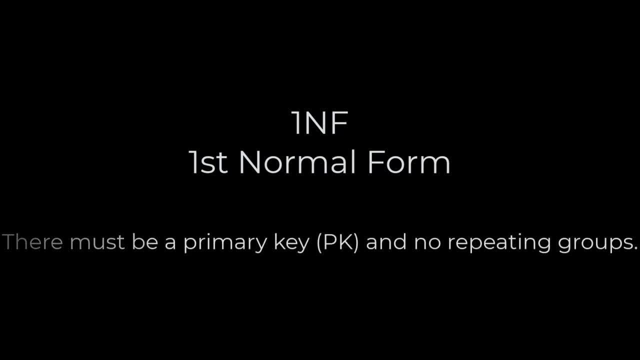 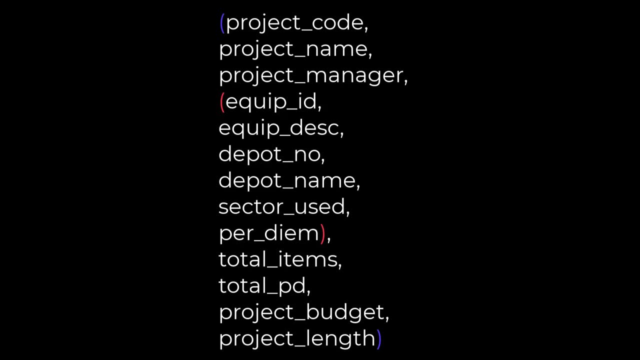 is to put the data into first normal form, where there must be a primary key and no repeating groups, and so currently this is kind of what the data looks like. there are two groups of data. the first group is in the blue brackets, that's sort of like the project, and then 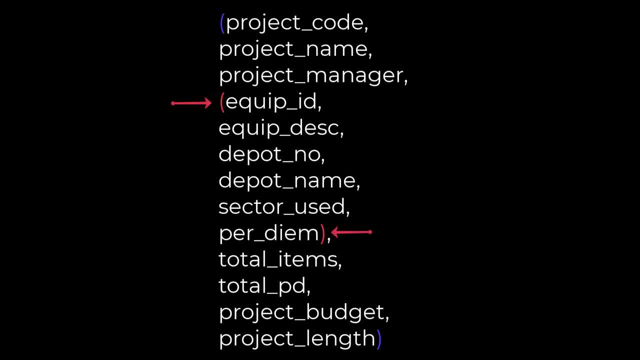 the equipment list on each project that's in the spreadsheet is in the red brackets there and that is sort of a repeating group, and you can see that the columns in the repeating group obviously seem to work differently than the columns in the project group. and so to take a closer inspection, 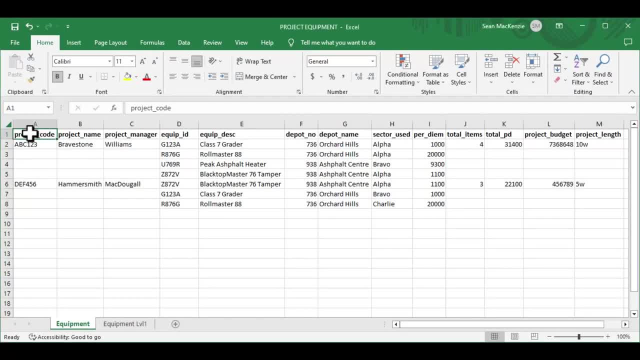 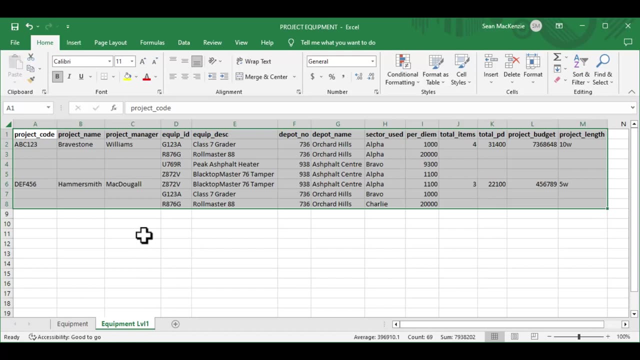 we can actually go to our spreadsheet here and we'll copy this over. i'll make this spreadsheet available to you on my downloads page and i'm just going to paste it into another another worksheet here and we'll change this data to conform to first normal form, which is: 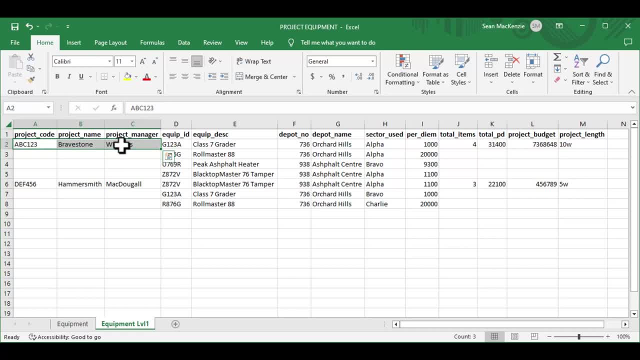 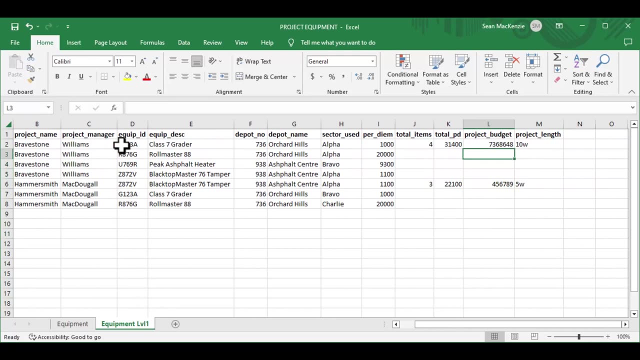 now we can split those two groups, the project and the equipment, into two tables or we can do a copy down which will satisfy. that will satisfy first normal form as well. it's not going to be the best for our database because we're going to go further, but we want. 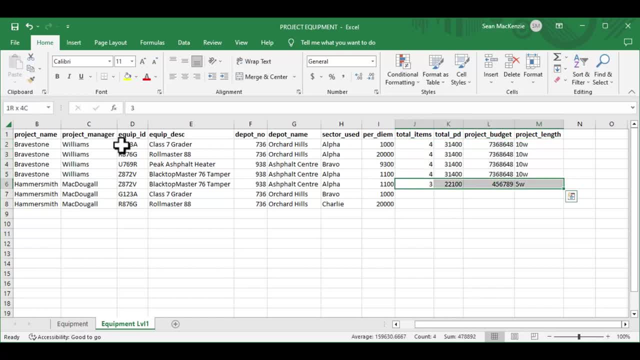 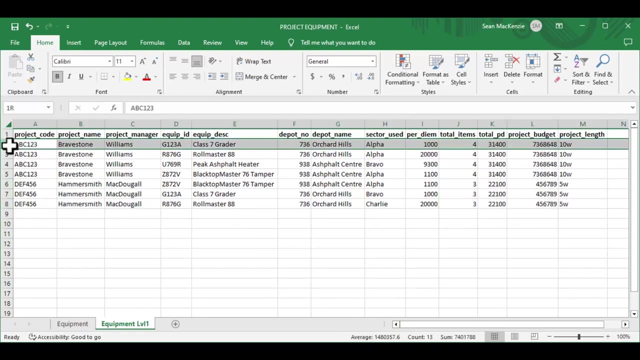 to first get our data into what we call first normal form, and so that would look kind of like this, where we, you know there's no repeating groups with empty spaces, there are just another first normal access usb, or have aavana called end machine. you can change that if you want to, you can celery it if you make change here to session. 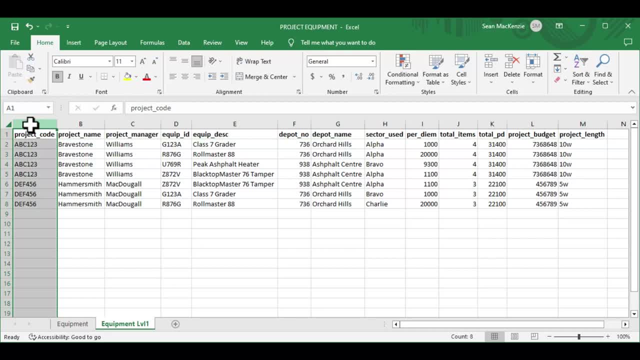 but i just wanted to show that thetrad Пол sitting, that little circle here by the end looks pretty like a piece of black daw né знаю gum handles and you can see we have the keyfile on the left side of each row, all the way back, all the way to start. we have to go back pretty late, but we're going. 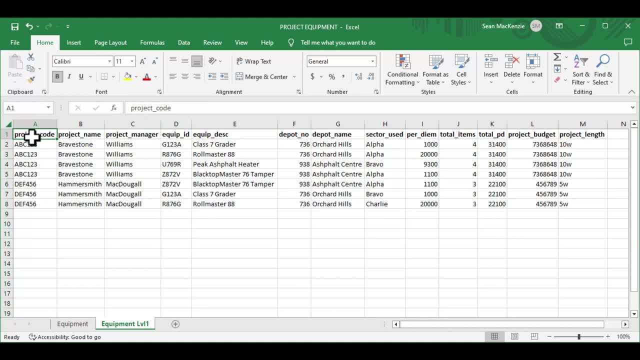 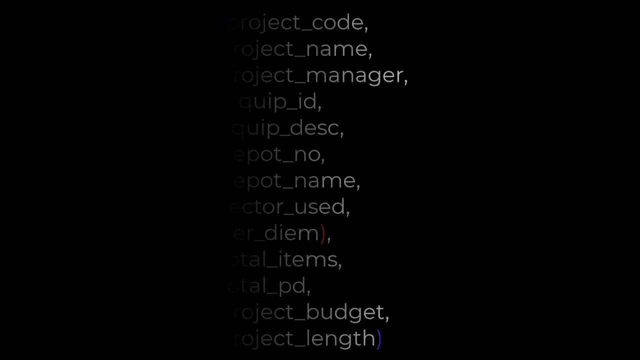 to go through the way that students do it, to see how you fit in with each row, the keyfile, which is that on the left side of each row, the keyfile here is id. it will uniquely identify every row in this table, and so, by doing the exercise we just did, 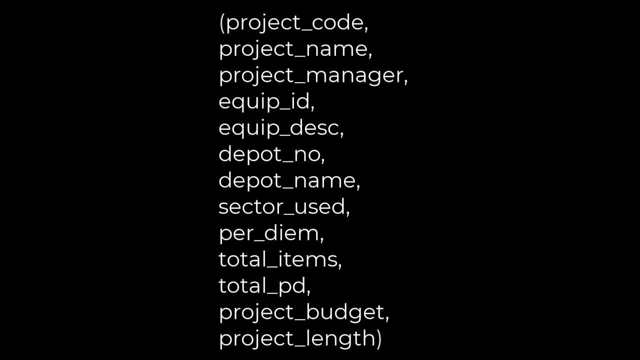 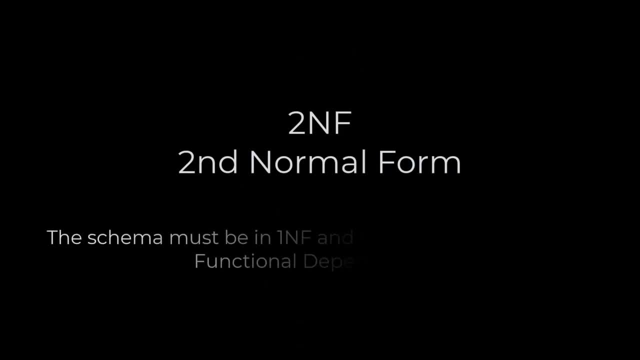 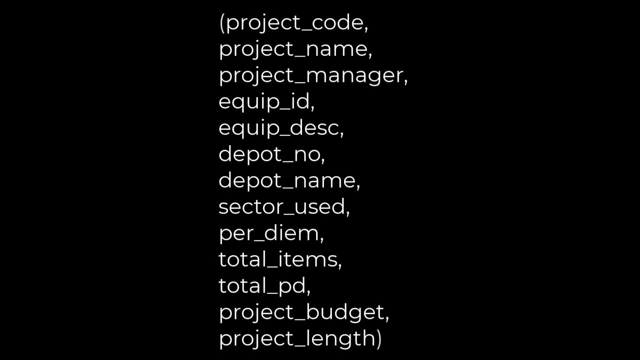 we're actually going to remove those red and blue brackets and we have one table which is first normal form. now for second normal form, we need to have a schema that is in first normal form and there are no partial functional dependencies, and by looking at this data i can see that there. 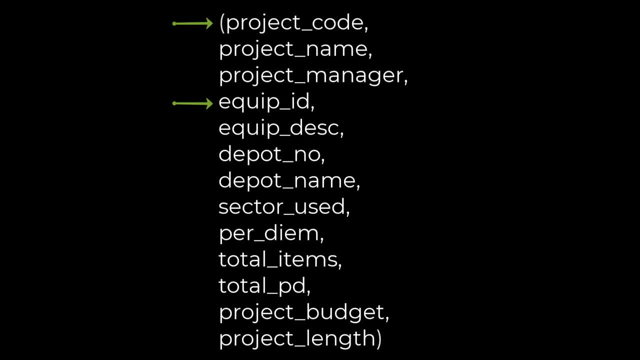 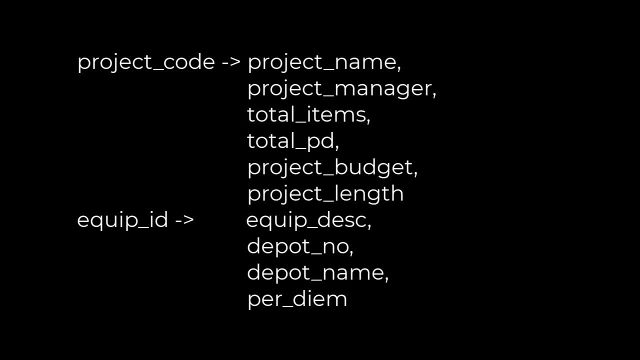 are two ids- the two ids that uniquely identify our records- but each of those has a list of fields that really only depend on that one key, and so those are called partial functional dependencies, and we can eliminate those by splitting the data for each of those keys into their own tables, and so that might look like something like this: we have project data. 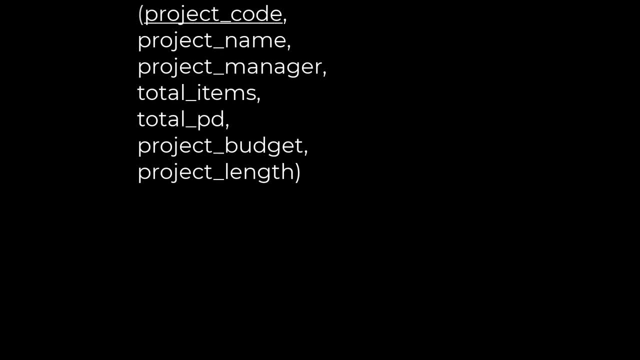 in this table and then we might have the equipment data in another table, which makes sense according to what we saw our dependencies were, but in this case we had leftover columns and we also have a relationship between the project and equipment data and that goes into a third table, which we can see here, that has project code and equipment id as well as the. 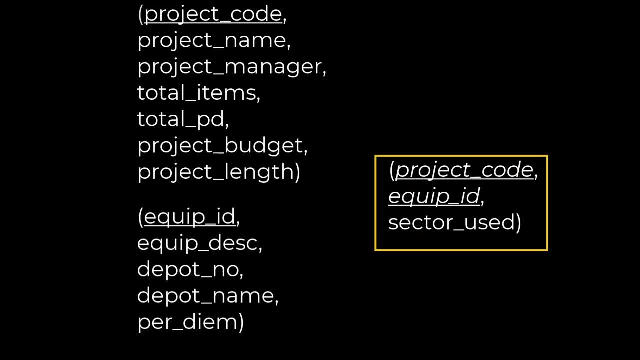 sector used, and this kind of table is known as a junction table or sometimes is called a transaction table, where you you can see the many to many relationship between the project code and equipment id fields and so you can see that sector used has been put on there. but this is typically where 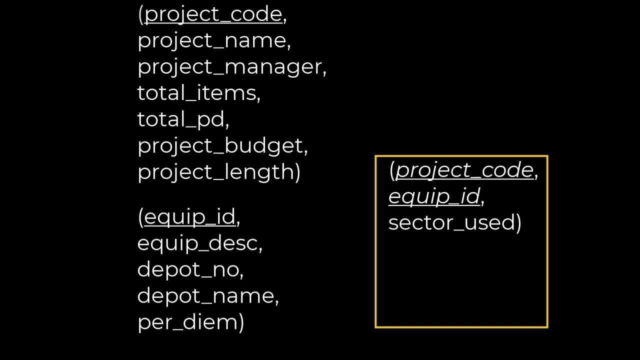 you'll add a whole bunch of information or fields in your table about that particular time, in this case that the equipment is being used, and more detail about that time that it's being used, and that's very, very handy and you can see how flexible this has suddenly become, because now we can have the same equipment. 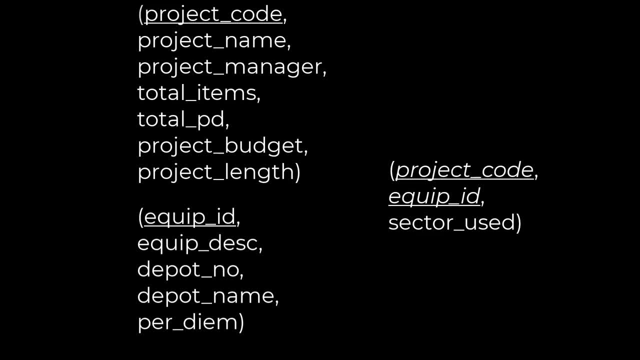 being used on many different projects, or many different projects using many different kinds of equipment over and over again, and it makes it for a very stable way to store lots of information about this particular scenario, and so at this point i will draw your attention to the underlying fields, just to remind you that those are primary keys. so the project 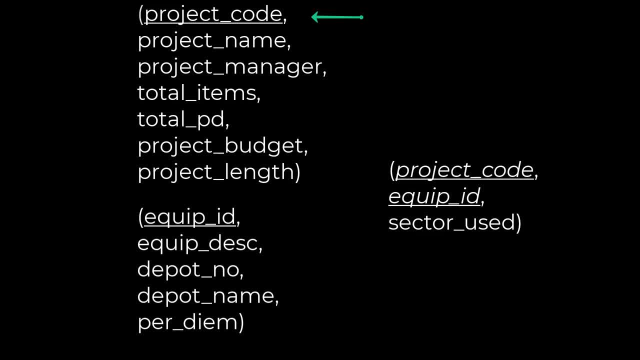 code is the key for the project table, the, the equipment id, is the primary key for the equipment table, and then the combination of the project code and equipment id together is used as the primary key for the uh, the table that's going to have the instance where a particular equipment. 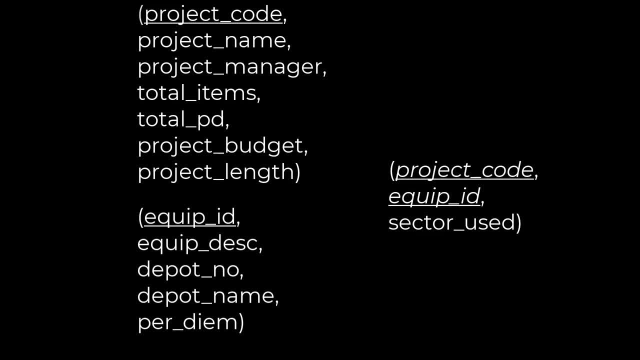 was used on a project. we haven't named them yet, but take a look at those fields that are in italics, and the italics denote that those are foreign keys, and so those are foreign keys. so you can see that that new table we created has a primary key that's made up of the two keys from: 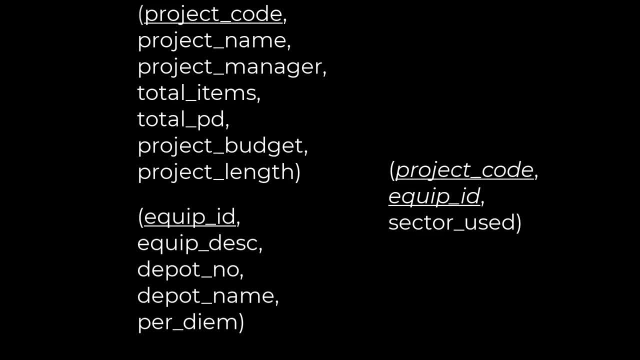 the other two tables, and so now that we have a table, that is just about the time that a piece of equipment was used on a project and it's different from every other time. then you can store other information, you know, like the driver, and all kinds of other things that are related to. 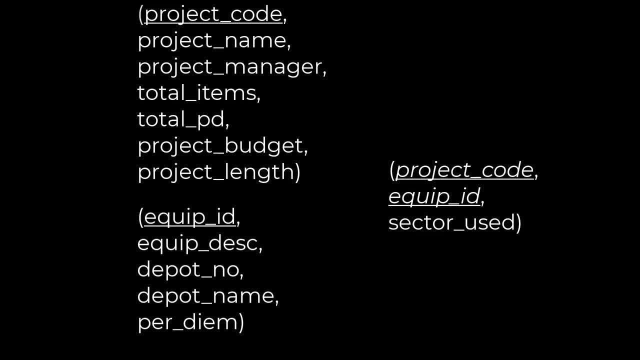 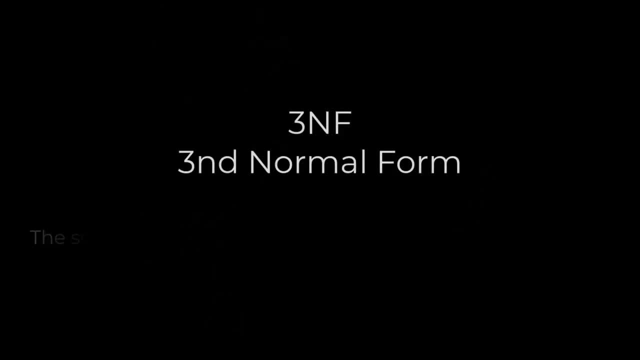 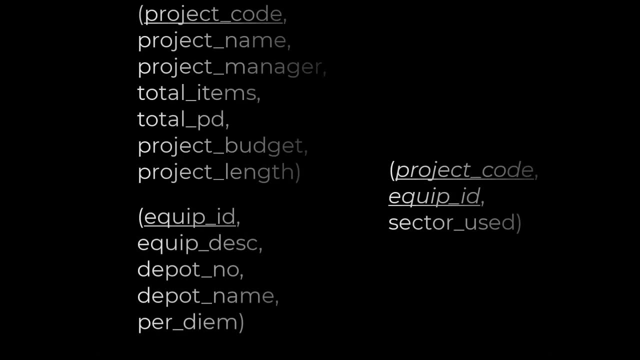 only that time that that that piece of equipment was used on a particular project, and so that gives us second normal form. and now we can look at third normal form, which means that the schema must be in second normal form and there are no transitive functional dependencies. and so, going back to our data, we can see that we do have a transitive 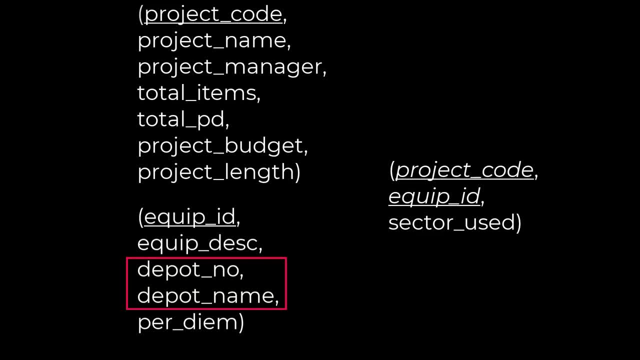 functional dependency, which means that there's a field or an attribute that actually is determined by another field in the same table, and so in this case we have a depot name which depends on the depot number and it never changes. they always have to be in sync, and so you can kind of think. 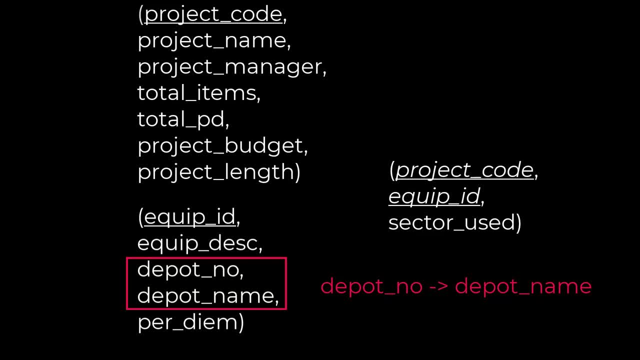 of these as as lookup tables. if you're an application designer, usually it'll be lookup tables, where you don't want to store the description of a lookup item in your table as well as the id. you just want to put the id in there and then, when you do a query, you bring. 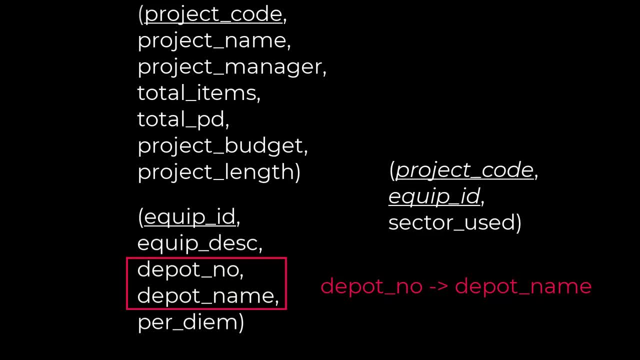 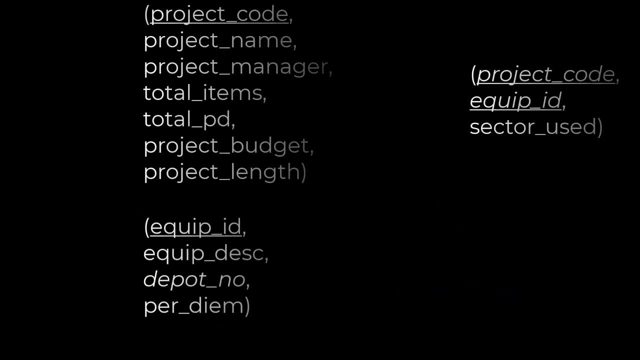 everything together to display it to the user, and so we want to eliminate all of the transitive functional dependencies from our tables, and what we might see would be something like this: where we remove that depot name from the equipment table and then put all of the depot information into another table, and not only